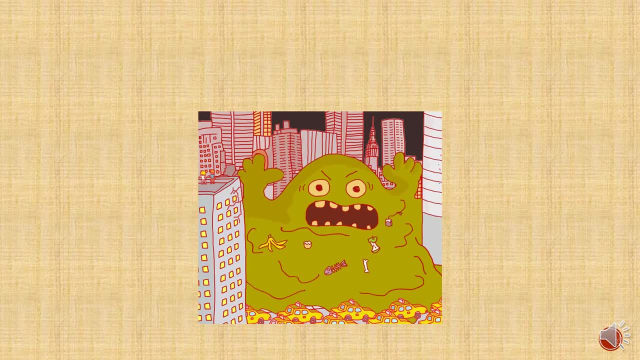 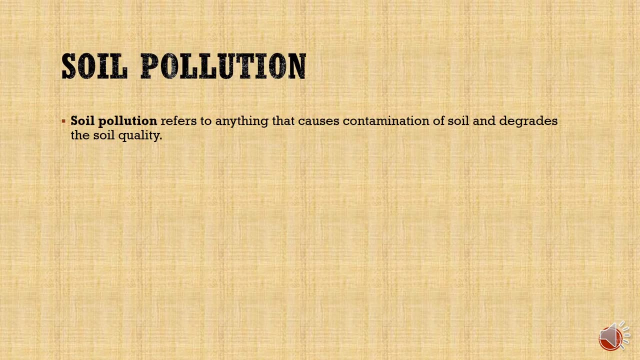 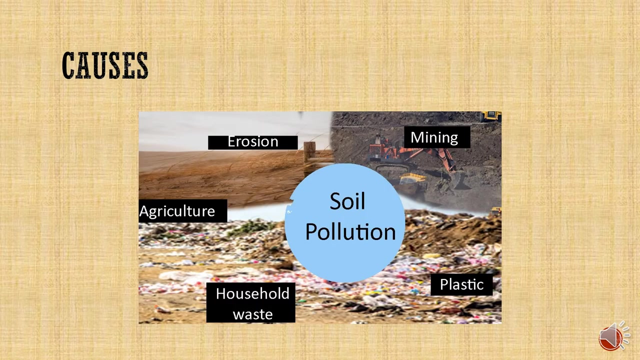 buried. When these wastes are buried, it causes immense soil pollution. But what is soil pollution? Soil pollution refers to anything that causes contamination of soil and degrades the soil quality. There are various causes of soil pollution, but the greatest cause is agriculture as it. 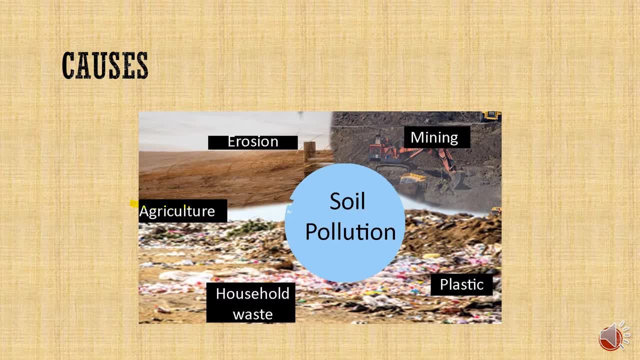 uses a lot of pesticides. Then there are mining activities. In mining activities, a lot of debris is littered over the surface, And then there are also overcrowded landfills, industries, construction activities, nuclear waste, sewage treatment, household plastics and erosion. 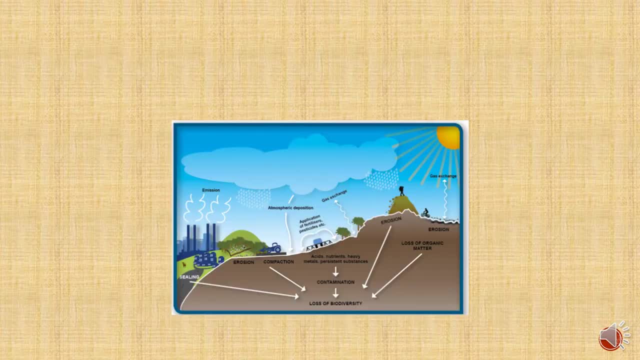 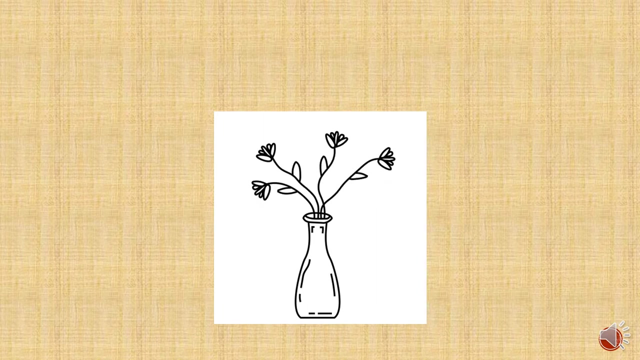 of land. Other pollutions are also contributing towards soil pollution, such as water pollution, air pollution. There are many causes behind. also, We often see that plants are wilting, animals are dying and climatic patterns are changing. So this is the effect of soil pollution. 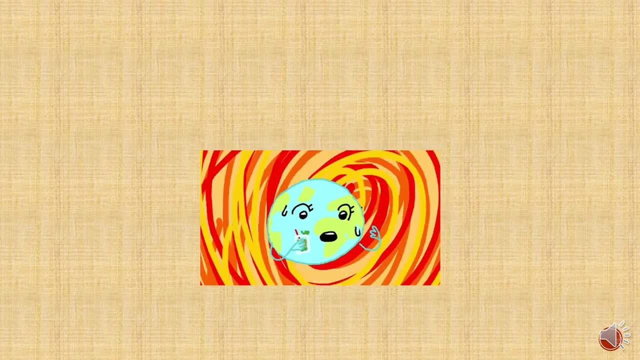 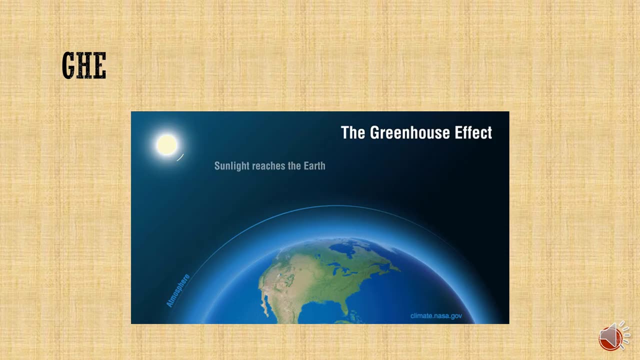 There is change in climatic patterns, also harsh winters and harsh summers. This is as a result of soil pollution. There are various environmental impacts. because of deforestation, hoping, the tree cover is compromised And that leads to unbalance in fields. Hash burners нас release. 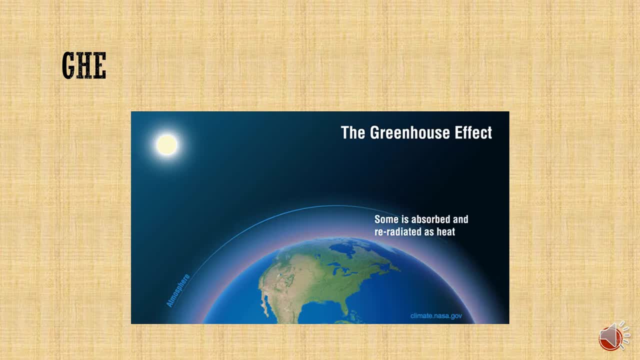 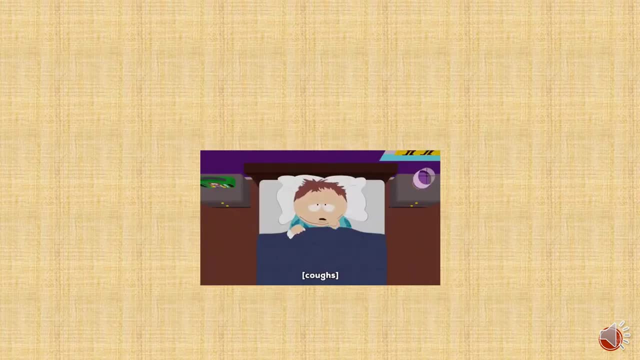 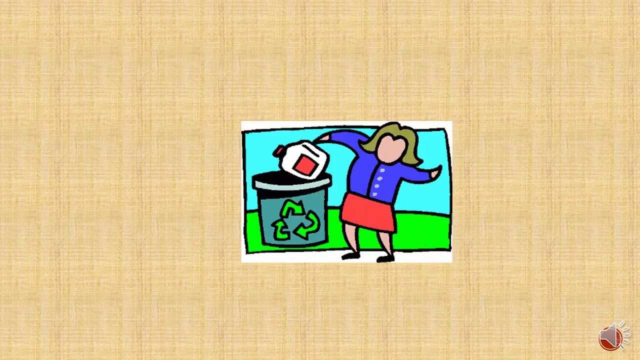 the caused interference that is creating деforestation and as風 re travels nature cycle, leading to greenhouse effect. human beings are highly suffering from soil pollution, from respiratory disorders to various cancers because of toxic chemicals and pesticides. nothing is impossible in the world if we are. 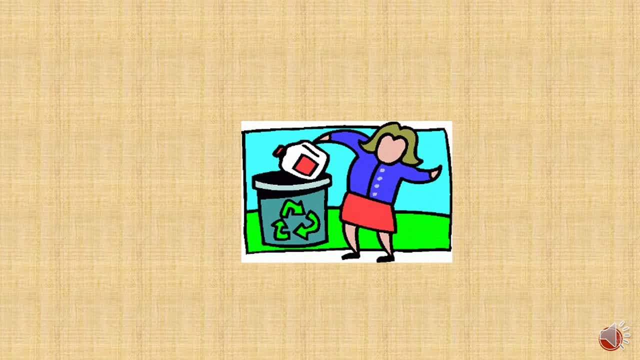 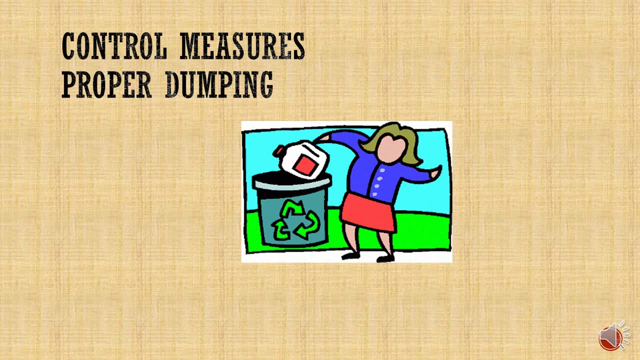 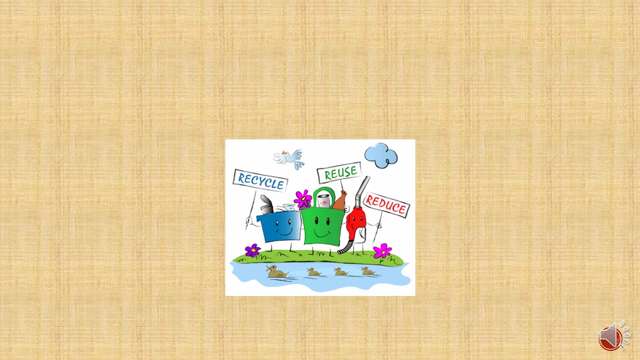 causing soil pollution. we can also control it. so there are many control measures which we can do to stop polluting our soil, for example, proper dumping of our debris and waste. we can also recycle, reuse and reduce our waste to minimize soil pollution. these are known as three Rs. we can maintain proper.